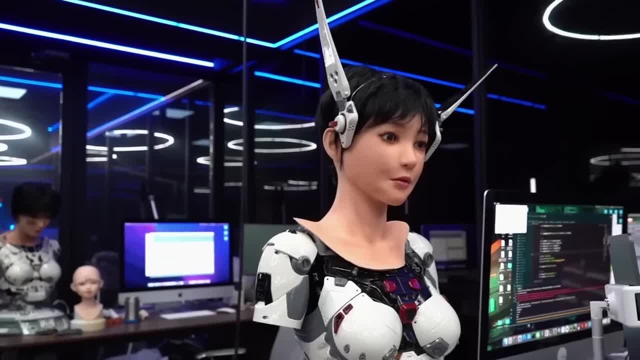 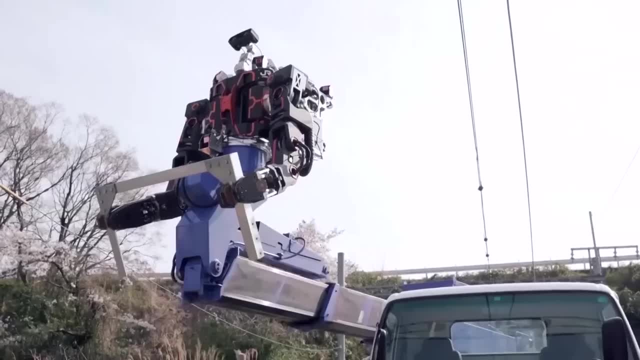 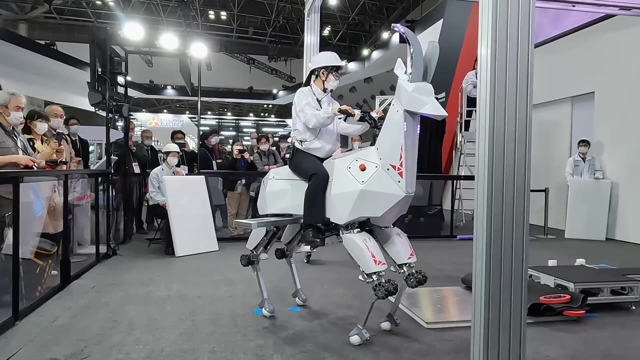 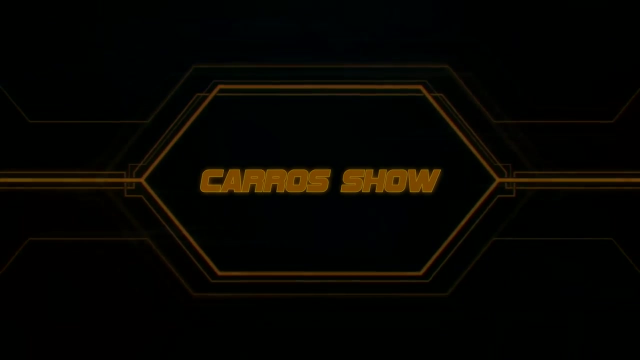 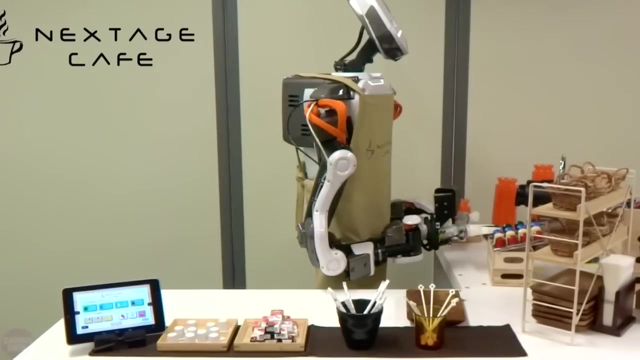 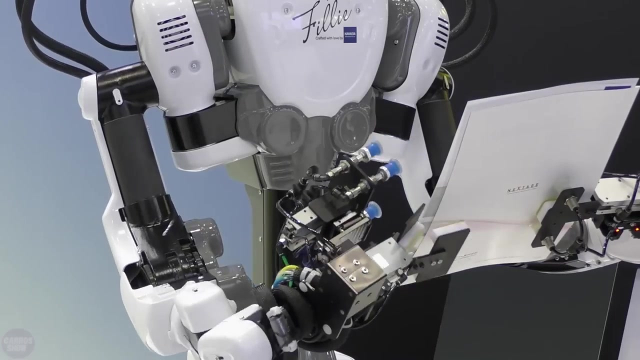 The Japanese company Kawada Robotics has developed one of the most advanced collaborative robots called Nextage. Nextage is a robot whose main task is to replace humans in monotonous works, such as on the production line. According to the manufacturer, the robot can collaborate with: 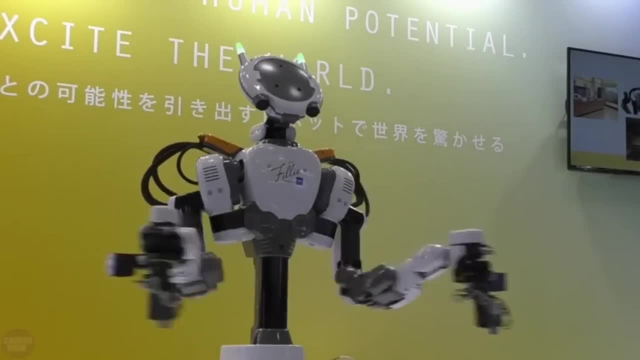 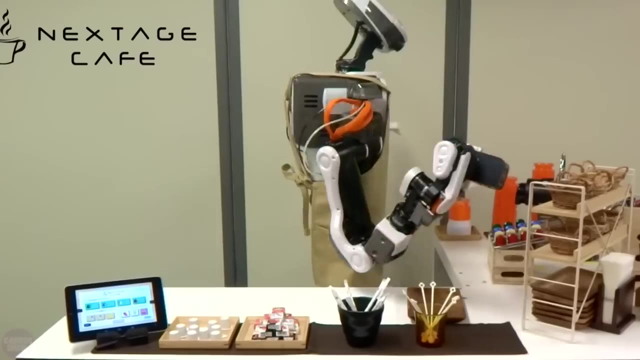 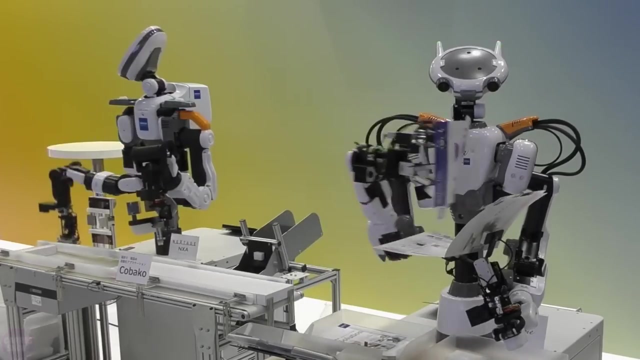 humans, other machines and use specialized tools. The robot's torso weighs only 29 kilograms, while its base is as heavy as 130 kilograms. As for its height, it is adjustable and can reach a maximum of 170 centimeters. Nextage is capable of lifting objects weighing up to 3 kilograms. 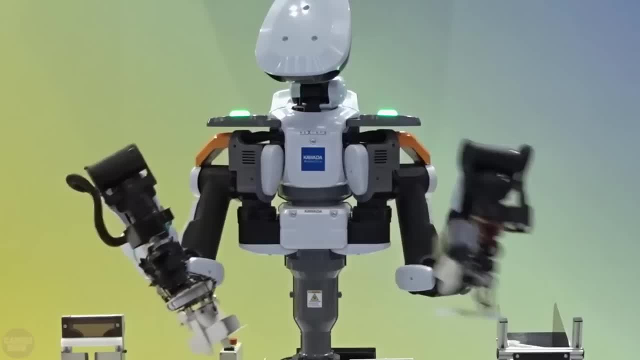 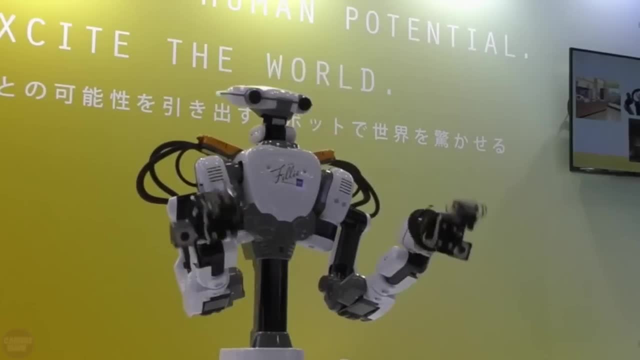 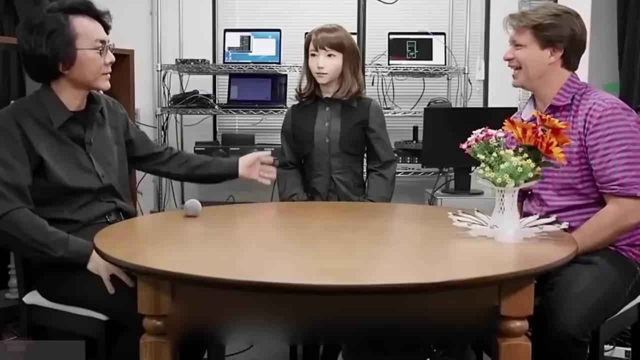 The robot is designed to work in factories and other production lines. It can be controlled using a tablet with special software that can be quickly customized for specific tasks. Professor Hiroshi Ishiguro from Osaka University gained worldwide recognition in the field of robotics thanks to the ultra-realistic android robots he and his team created with the most. 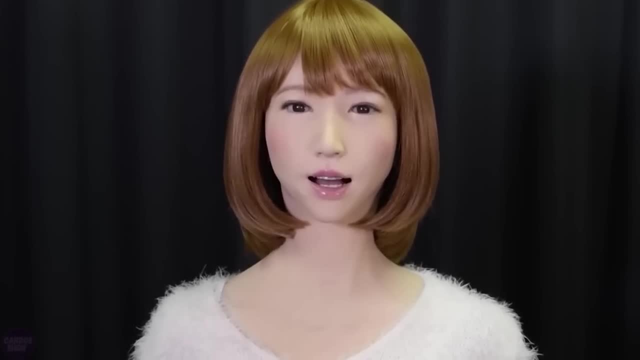 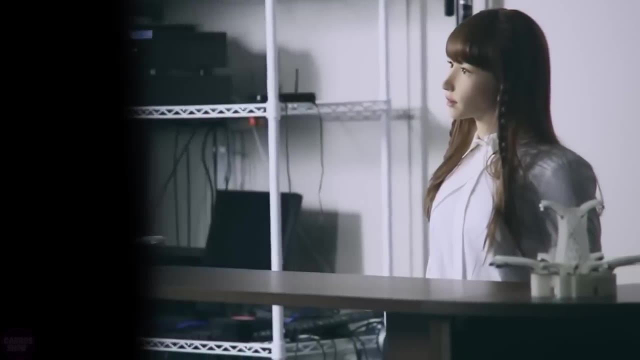 popular one being the robot Erika. Erika is a humanoid robot functioning due to a synthetic organism with an electronic brain system. The robot's body can have various organs of real humans which are indistinguishable, both in appearance and functionality, from real ones. 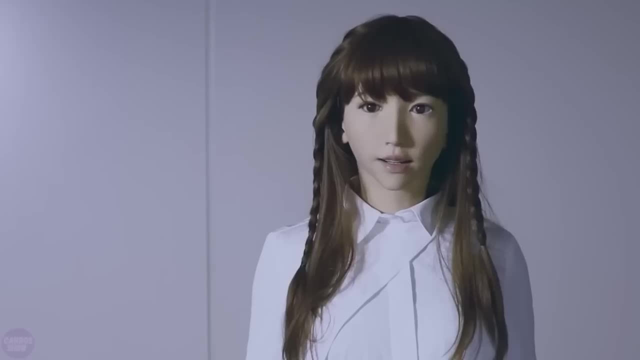 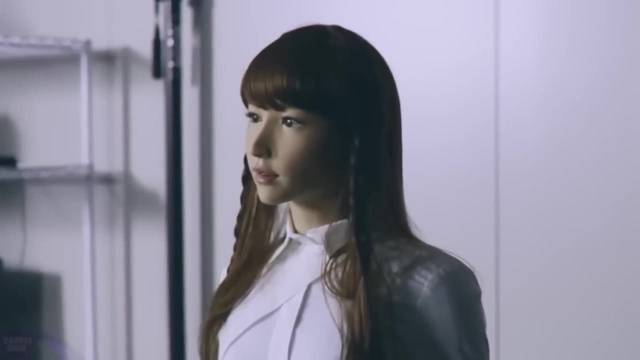 According to scientists, a gynoid is a humanoid robot woman, essentially the same as an android, but of the female gender. Creating a new android, Professor Ishiguro's team not only provided the robot with new eyes, ears and other more realistic parts, but also equipped it with 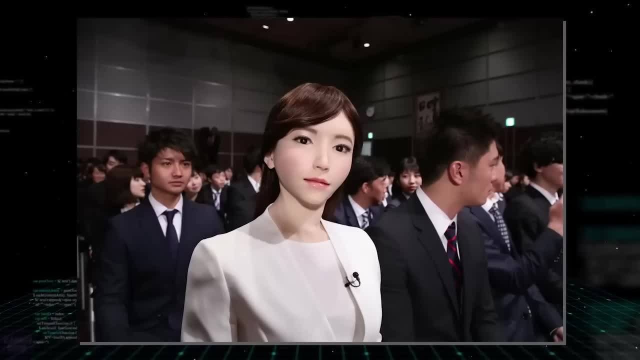 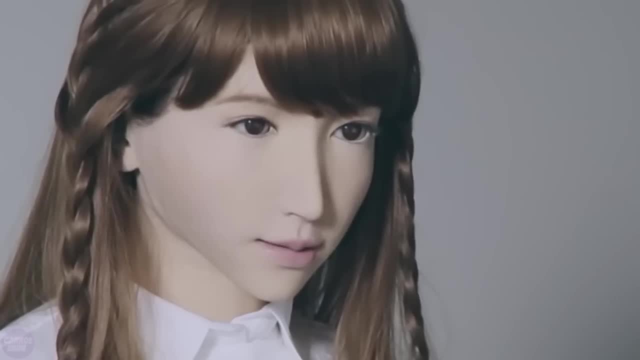 conversational capabilities. Despite all the efforts of roboticists, Erika still looks a bit wooden compared to living humans. However, the robot can engage in casual conversations on a range of simple topics and answer questions like what is your hobby? Researchers recently announced 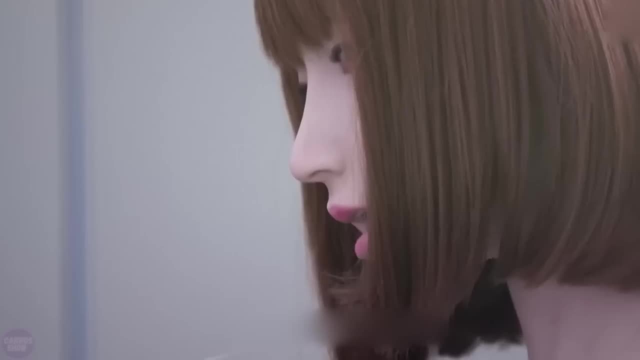 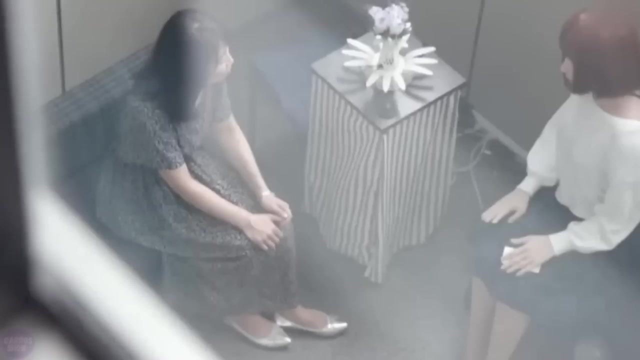 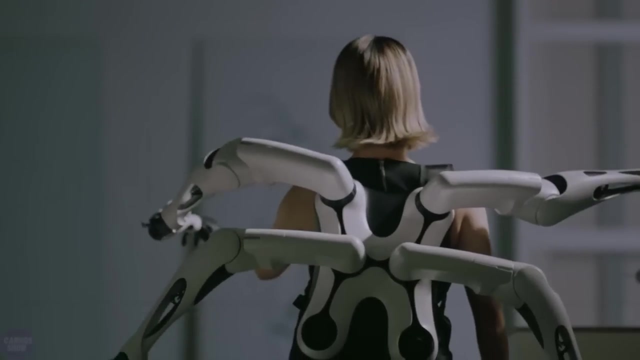 plans to connect Erika to an artificial intelligence system enabling her to freely converse on various topics. It's intriguing to wonder whether Erika will surpass the limits set by humans and potentially lead to a machine uprising after being connected to artificial intelligence. Engineers and designers from the University of Tokyo have developed a robotic backpack called 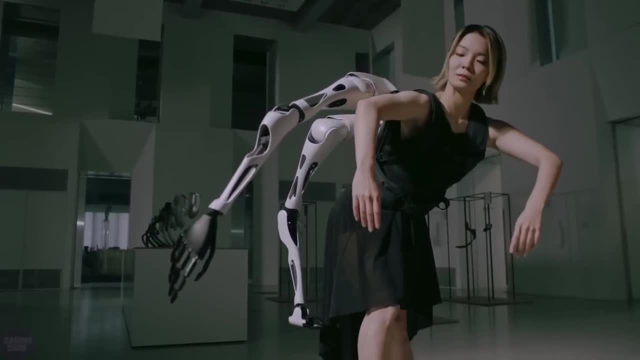 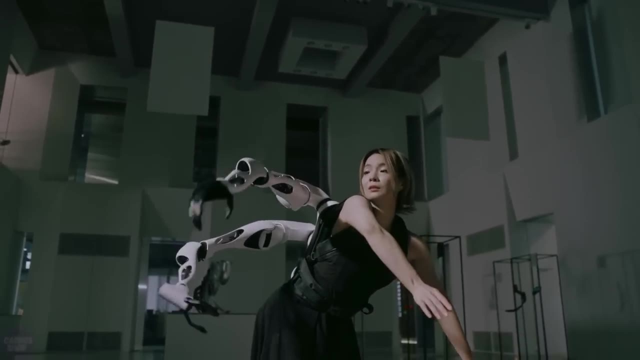 Jizai Arms, which allows connecting up to six mechanical arms. This device attaches to the torso using several straps and the hands of the arms can be interchangeable. The user can choose between human-like hands and grippers. The robotic backpack weighs 4.1 kilograms without the robotic 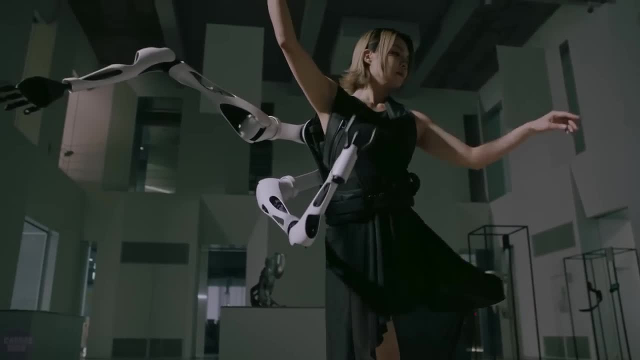 arms. When the robotic arms are connected, the weight of the device increases to 14 kilograms. The arm movement is the same as the arm movement of a human. The arm movement is the same as the arm movement of a robot. The arm movements are controlled remotely using a special setup which is a scaled-down. 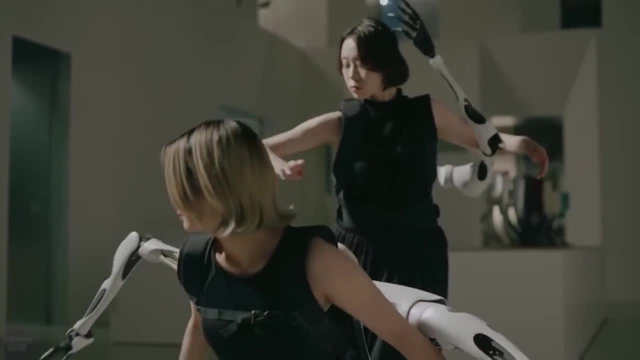 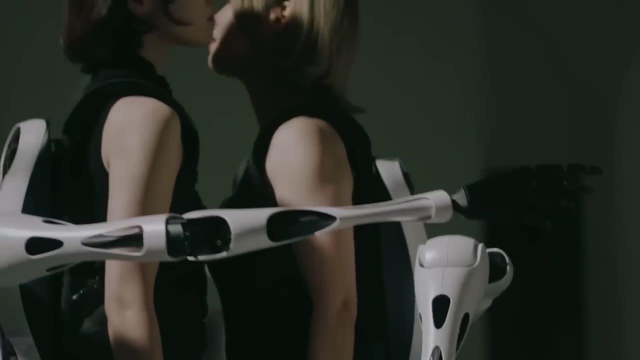 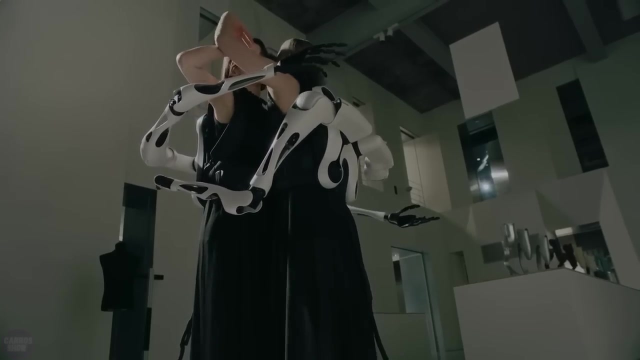 replica of the device itself. Currently, controlling the arms through the robotic backpack presents certain challenges. Sometimes the cooperation of multiple operators is required and it is impossible to use the device without the assistance of others. This is the main problem that needs to be solved. However, in the future, with the development of neural interfaces, it may be. 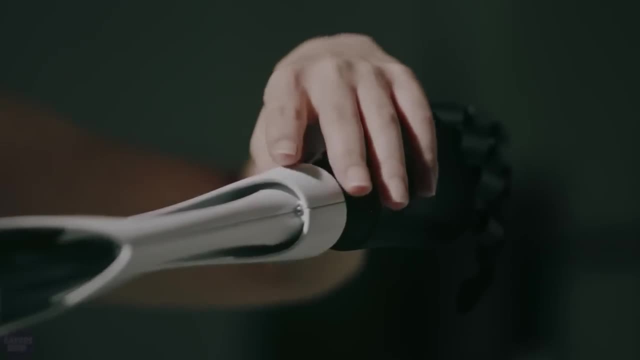 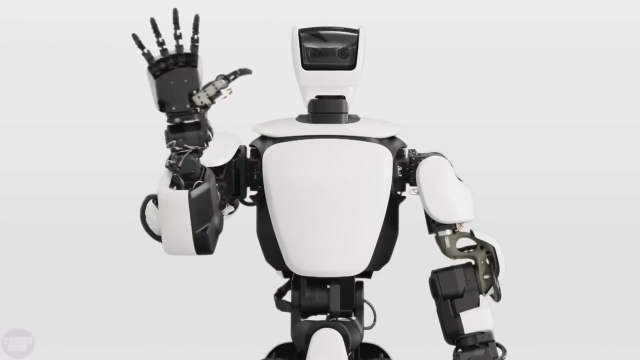 possible to achieve mind-controlled operation, allowing the user to control the robotic arms as if they were their own. The robot's movements are controlled by a human operator using the Master Maneuvering System module. Engineers at Toyota have developed a humanoid robot called THR-3.. Since its creation, the robot has 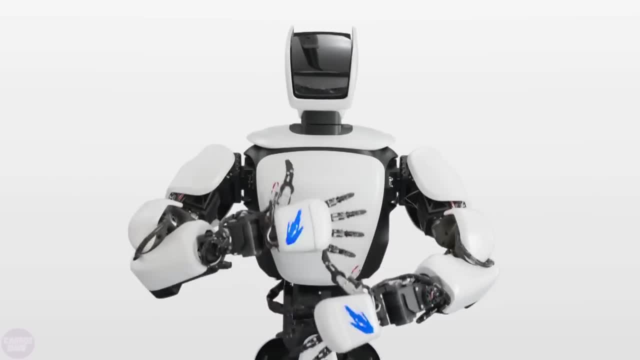 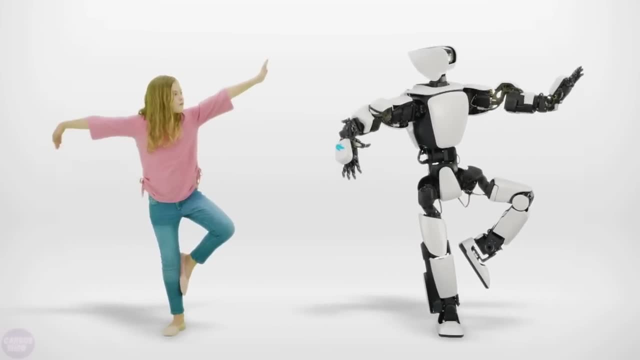 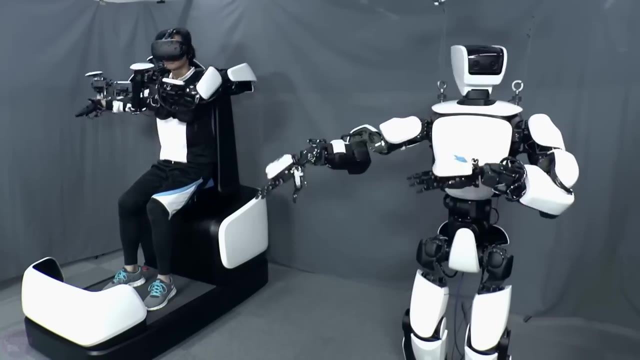 undergone numerous updates and improvements, significantly increasing its functional capabilities. The robot's movements are controlled by a human operator using the Master Maneuvering System module. The operator received tactile feedback and the image transmitted from the robot displayed on a virtual reality headset. HTC Vive, Special gloves and servo motors are also used in. 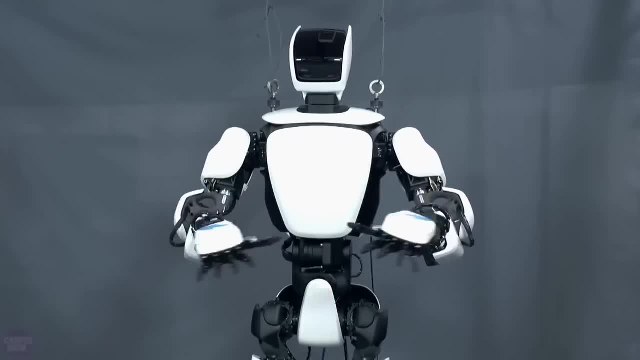 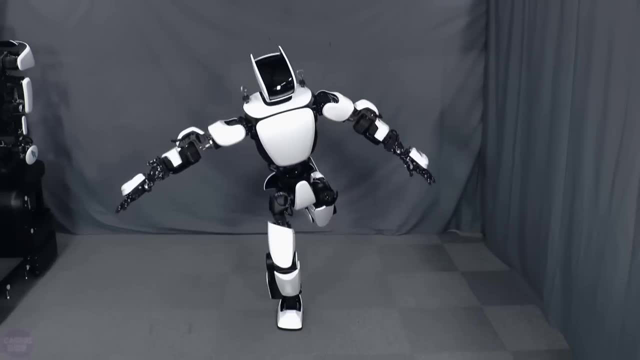 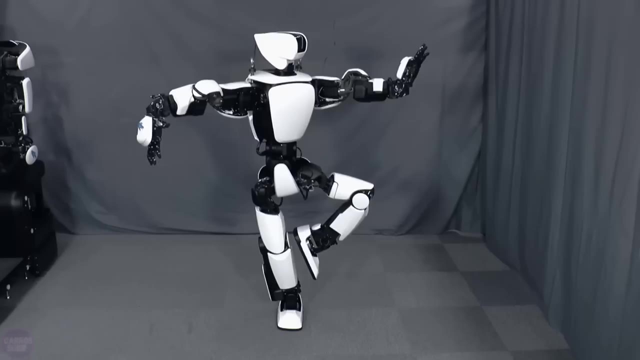 order to enable the operator to control the robot instantly, with precise movements and applied force. The robot demonstrates excellent balance, including the ability to stand on one leg and perform various movements. Toyota's robot stands at approximately 152 centimeters and weighs about 75 kilograms. While it serves as a test platform, the ideas and capabilities implemented in it can 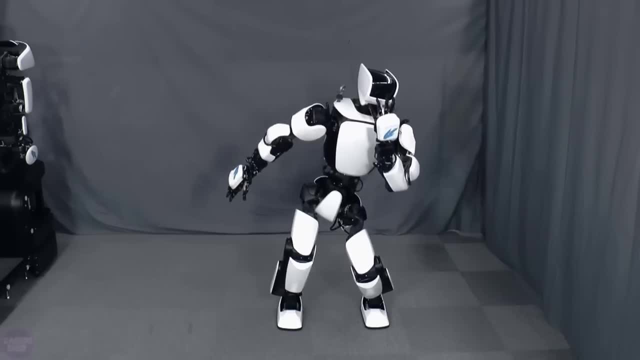 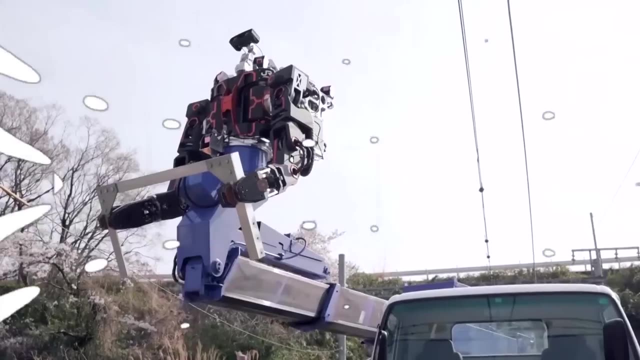 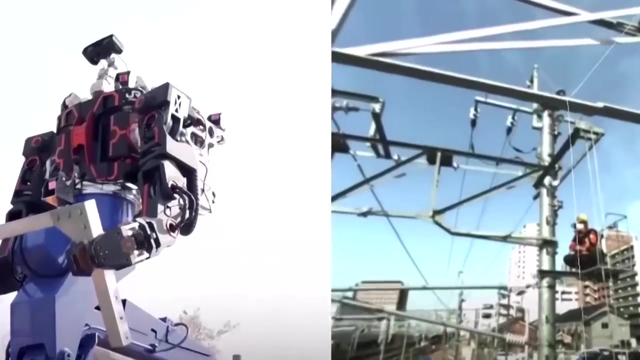 be used in devices for home use, medical facilities, construction sites, areas affected by natural disasters and even space in the future. The Japanese robotics company Jinki Itai has attracted significant attention with its unique heavy machinery, a humanoid industrial robot that can be remotely controlled by a human. 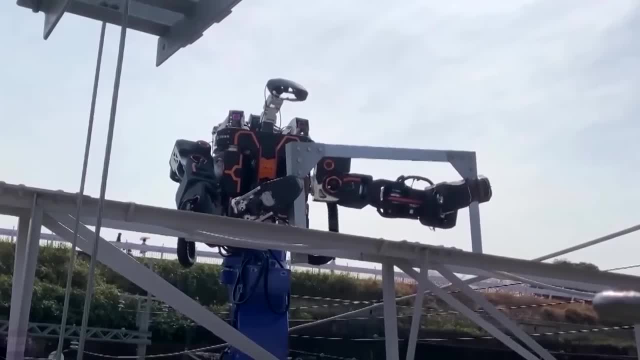 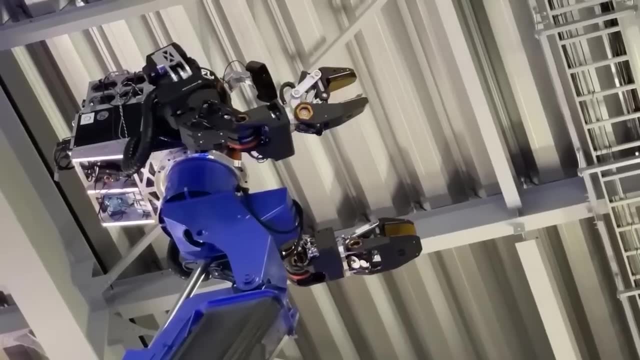 The Jinki humanoid robot serves as an example of human-machine integration. The robot has a head, torso and two arms that extend upward from a specialized cabin resembling an excavator's cockpit. Designed for technical maintenance tasks in various fields, such as repairing railway tracks or replacing and repairing the railway tracks, the Jinki Itai has a 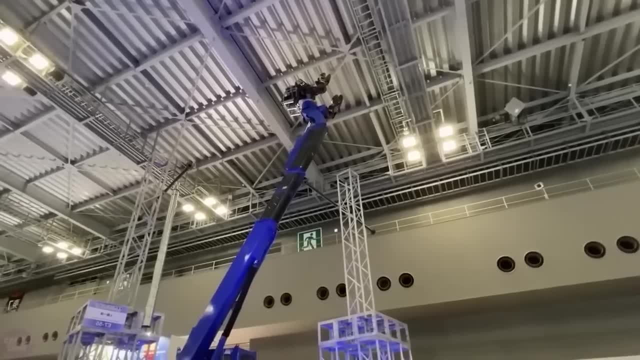 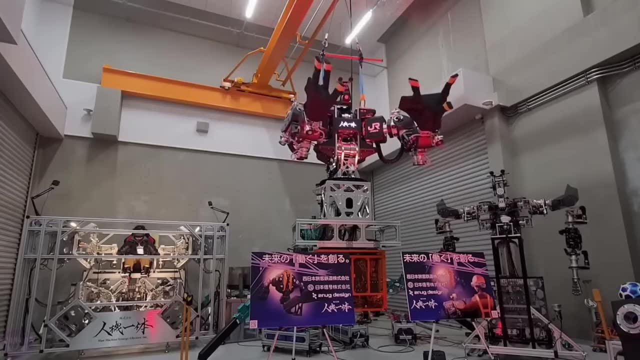 robot that can control the robot's arm movements. using technology developed by the company, The robot is capable of lifting and moving heavy loads such as steel pipes, plates or wires, and performs its tasks as effectively as a human, as it is controlled by a human operator. 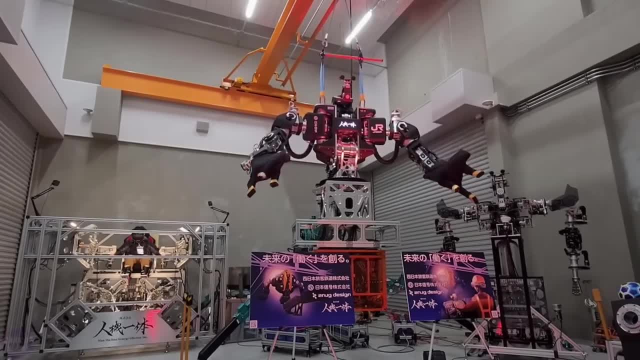 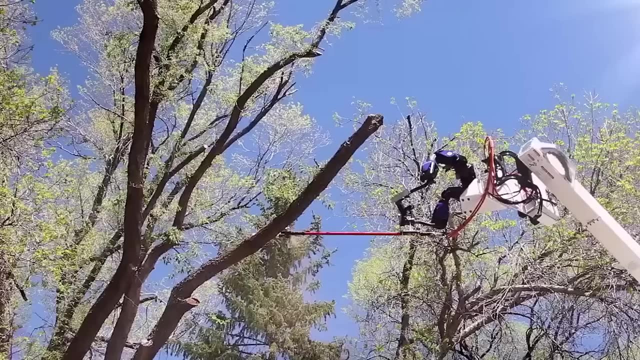 Jinki essentially replicates the movements of a real person inside the heavy machinery cabin. The operator wears special glasses connected to the robot's eyes, allowing precise control of the robot's arm movements using technology developed by the company. The robot is also capable of. 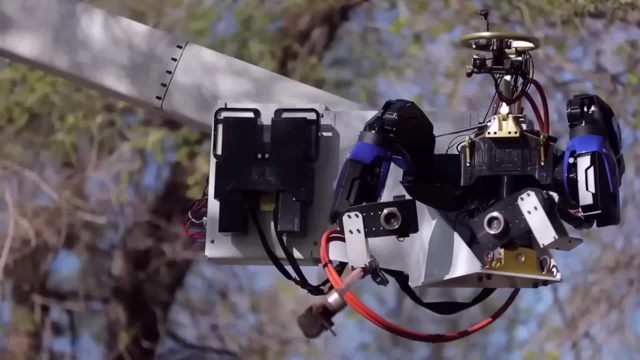 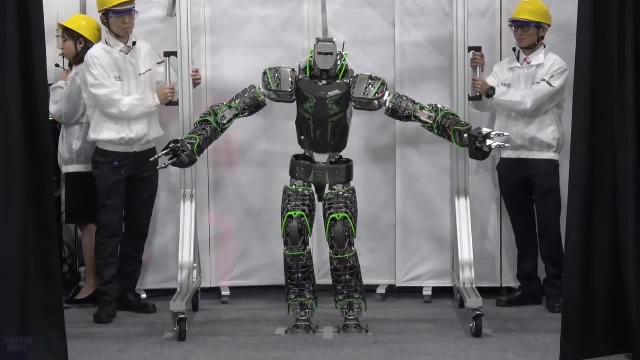 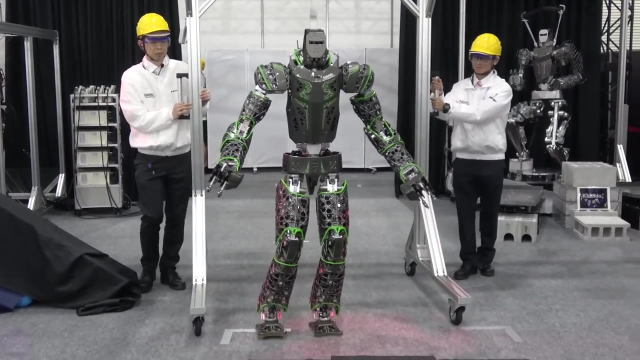 controlling the robot's arm movements using technology developed by the company. Can you imagine how humanoid robots are landing in places affected by natural disasters on a rescue mission, or where these robots take care of severely ill or elderly people? One of the few companies making significant advancements in this field is Kawasaki Heavy. 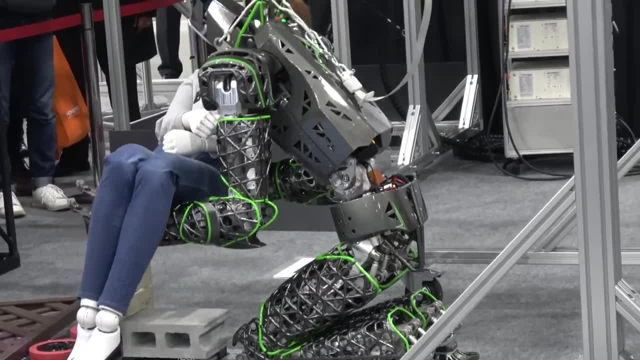 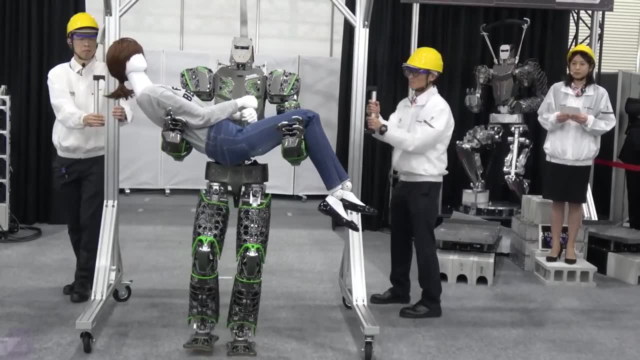 Industries, commonly known as Kawasaki. One of the company's most outstanding developments is the humanoid robot Kaleido, standing at 184 cm tall and weighing 85 kg. The robot is designed to work in dangerous areas such as collapsed structures, fires and natural 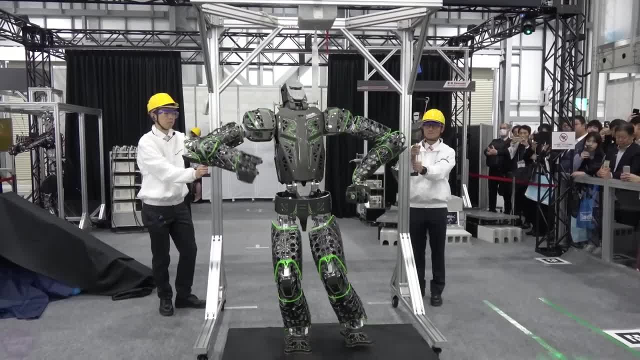 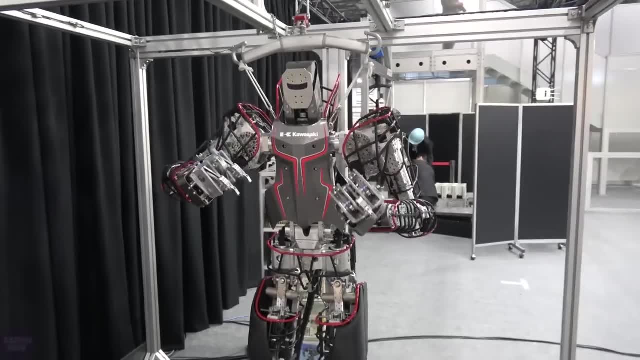 disasters. Developers assure that in the future, it could operate at the ocean floor or even in space. Its humanoid form enables it to use the same tools as humans. Kaleido is durable and easy to repair, making it a very interesting and promising innovation. 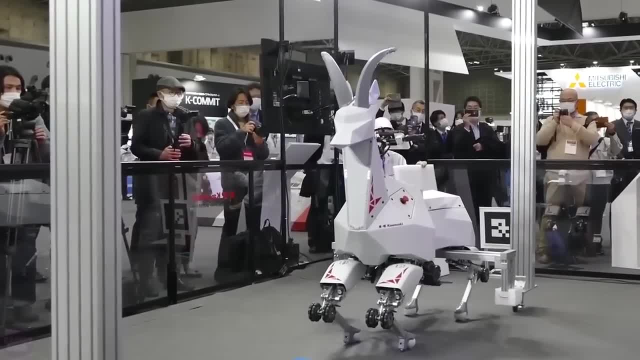 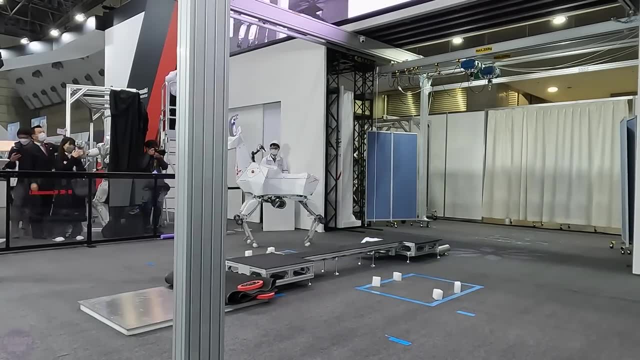 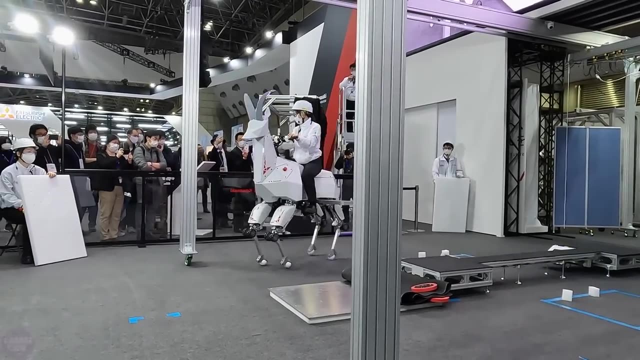 Why torture real horses when robots can be harnessed? Kawasaki recently showcased a robotic goat capable of jumping and carrying loads, officially unveiled at the 2022 International Robot Exhibition in Tokyo, which we covered in a separate video on our channel. BEX is an offshoot of the Kawasaki Kaleido program In its regular mode.